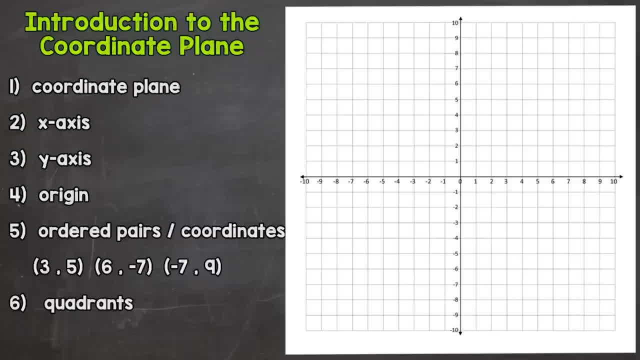 coordinate plane, And a coordinate plane is a two-dimensional surface so flat on which we can plot points, lines, curves, etc. Now, here on the right hand side of your screen, is an example of coordinate plane, And then number two and number three. this is what our coordinate plane consists of. It consists of: 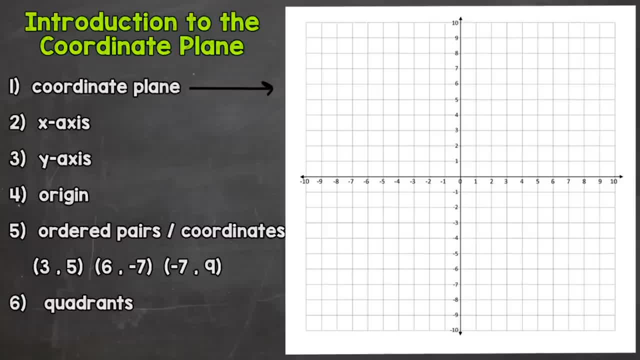 an x and a y-axis and it's very important to know the difference between the x and the y-axis. So the x-axis is the horizontal or side to side axis. So I'm going to come over to the right hand side of your screen and label the x-axis Again: x side. 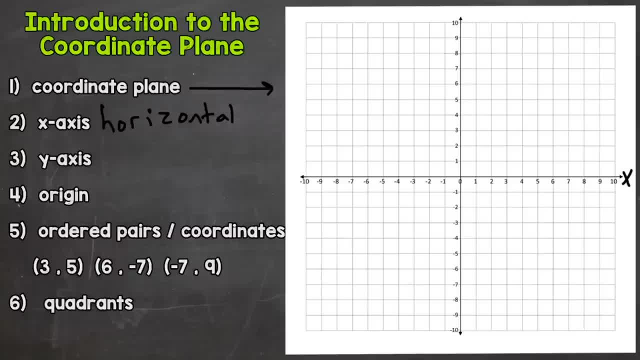 to side or horizontal. Now y-axis is the vertical or up and down. So I'll come to the top of your screen here and label that the y-axis. So again, x side to side, y up and down. Now number four and second grade. we have the origin, and the origin is where everything starts. 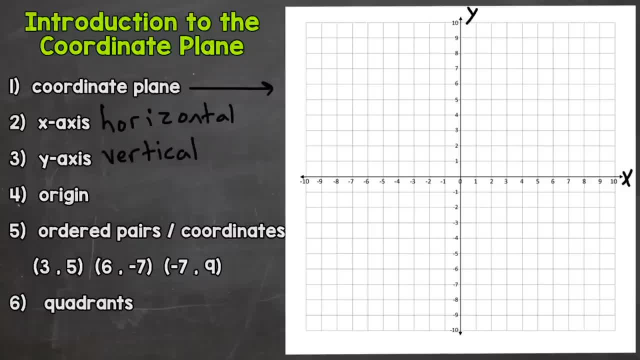 Our coordinate plane. when we plot points, we always start at 0: 0 and go from there. So I'm going to put a circle around the origin here: 0: 0.. So when we plot points, we always start there at the center and then go side to side and then upward down. 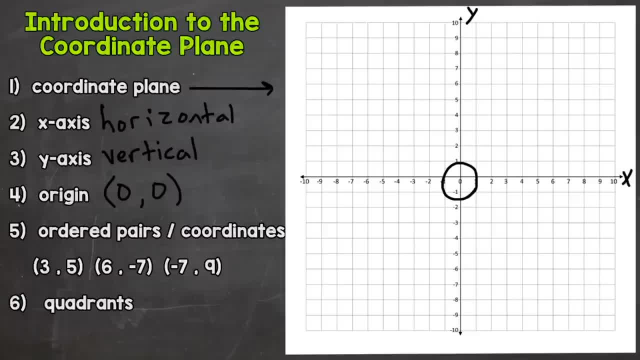 And we're going to go through here, through a few examples of those here. next for number five. So for number five, we have ordered pairs, slash coordinates, Now the two numbers within the parentheses. so for example, this three and five, that's an ordered pair, The. 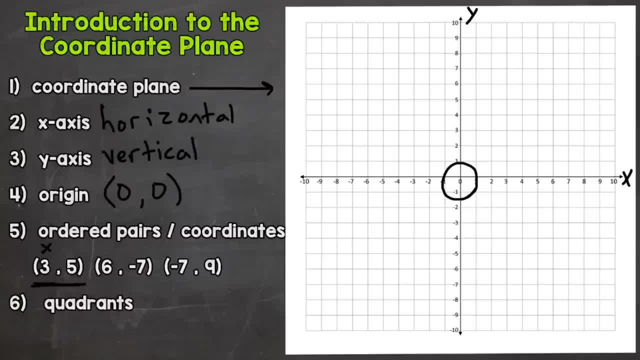 three is the x-coordinate and the five is the y. The x always comes first. You always go side to side and then up or down. So let's plot three, five. We start at the origin, in the center of our coordinate plane, and we go over three on. 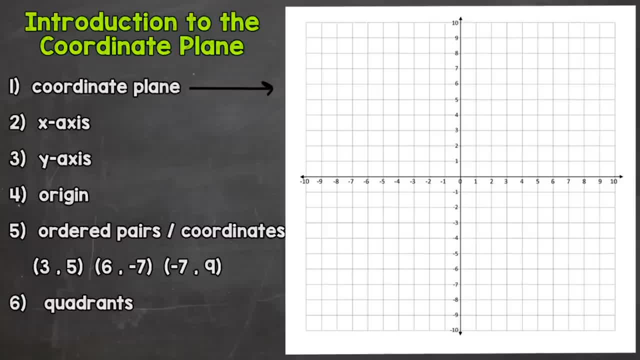 an x and a y-axis and it's very important to know the difference between the x and the y-axis. So the x-axis is the horizontal or side to side axis. So I'm going to come over to the right hand side of your screen and label the x-axis Again: x side. 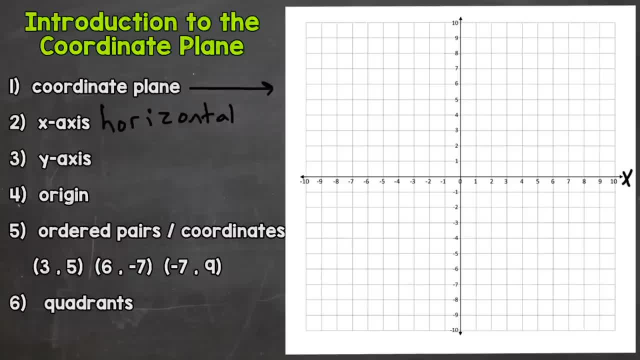 to side or horizontal. Now y-axis is the vertical or up and down. So I'll come to the top of your screen here and label that the y-axis. So again, x side to side, y up and down. Now number four is the explodingionen. What the y-axis shows is going to point towards where weάν. 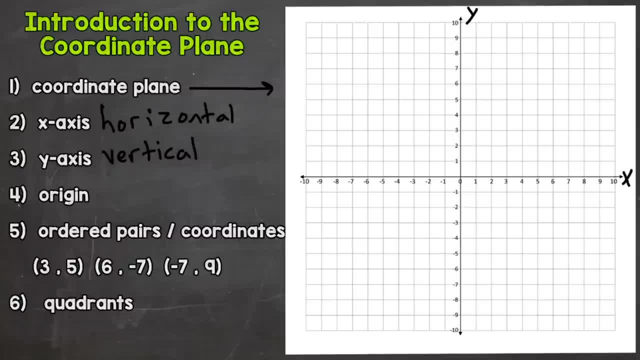 we have the origin, And the origin is where everything starts on our coordinate plane. when we plot points, We always start at zero, zero and go from there. So I'm going to put a circle around the origin here: zero, zero. So when we plot points, we always start there at the center and then go side to side and then evening. 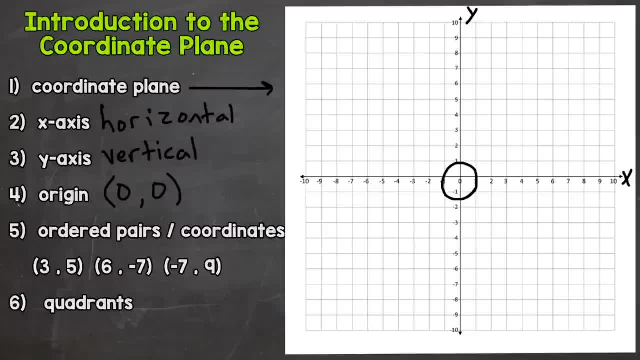 up and down In order to get to the point where we have our coordinates. And now, as I go game on here, we're going to" through a few examples of those here. next for number five. So for number five, we have ordered pairs, slash coordinates. Now the two numbers within the 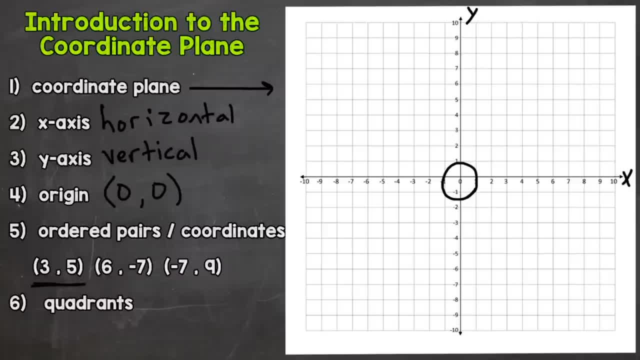 parentheses. so for example, this three and five, that's an ordered pair. The three is the X coordinate and the five is the Y. The X always comes first. You always go side to side and then up or down. So let's plot three, five, We start. 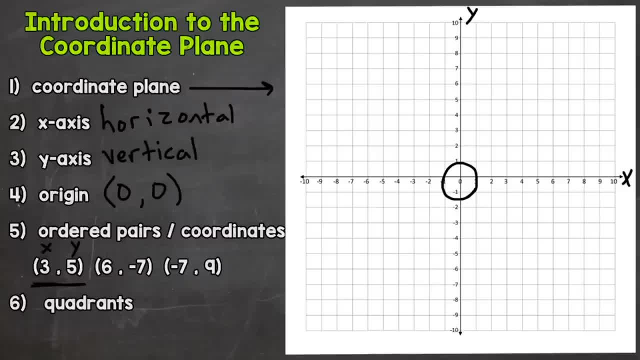 at the origin, in the center of our coordinate plane, and we go over three on the x-axis. Now that's a positive three, so I'm going to underline that there. So we go over three and then up to positive five. Now where those intersect, we plot a. 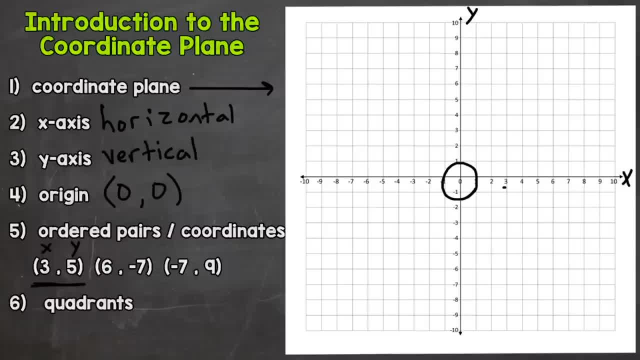 the x-axis. Now that's a positive three, so I'm going to underline that there. So we go over three and then up to positive five. Now where those intersect, we plot a point and I'm going to label that point, so we know exactly where we plotted that point. Now the second ordered pair six. 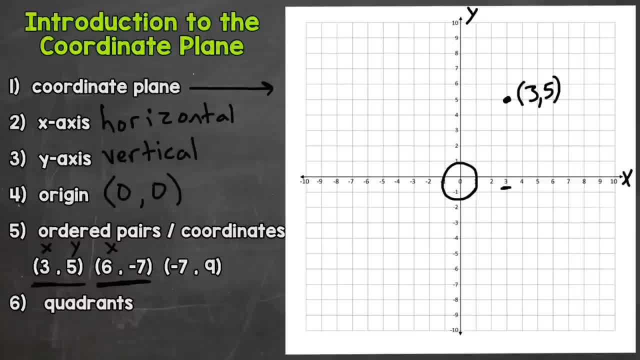 negative seven. So again, x always comes first, followed by our y-coordinate. So we would start at the origin, in the center. We would go over a positive six. Now, this time we're going to go down seven, though, because that's a negative seven, So over. 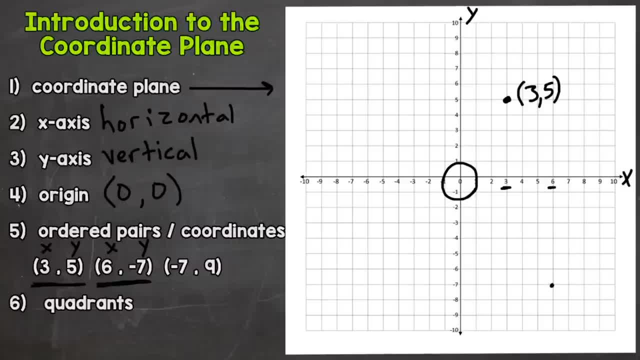 six, down to negative seven. plot a point where they intersect. I'm going to label this point as well. And then, lastly, we have negative seven, nine. So again, x always comes first, followed by y. Now, this time, we're going to go left of zero. 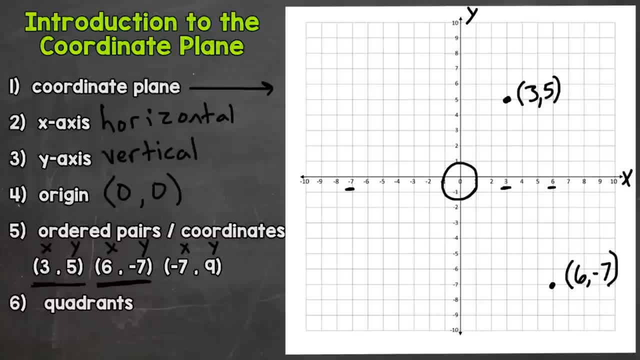 because that's a negative seven. So negative seven is over here, and then our y is positive, a positive nine. So we're going to go up, Plot our point and I'll label negative seven, nine. So again, always side to side, and then up or down. Lastly, we have quadrants. 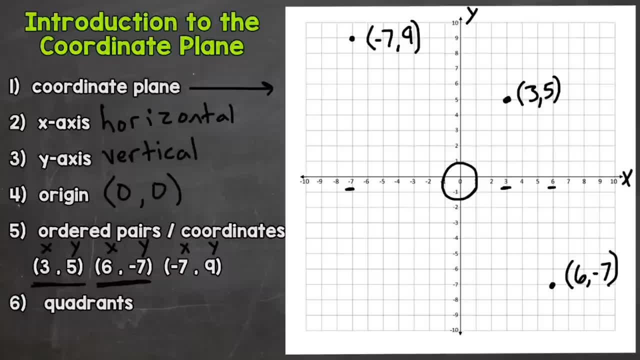 Now, if you look at your coordinate plane, there you'll notice that we have four sections: top right, top left, bottom left, Bottom right. So this three, five right here, this top fourth, this is considered quadrant one. I'm going to use Roman numerals here. Now I'm going to jump to. 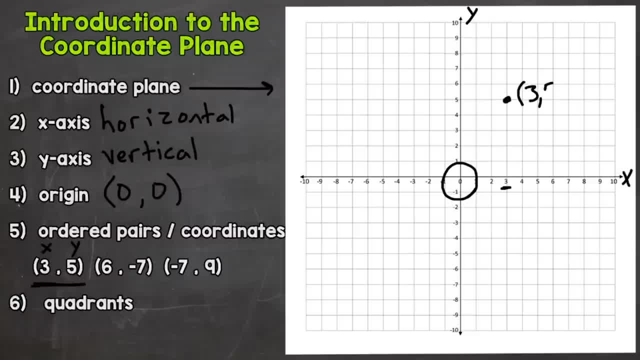 point and I'm going to label that point so we know exactly where we plotted that point. Now the second word: pair six negative seven. So again, X always comes first, followed by our y-coordinate. So we would start at the origin, in the center. We would go over a positive six. Now this: 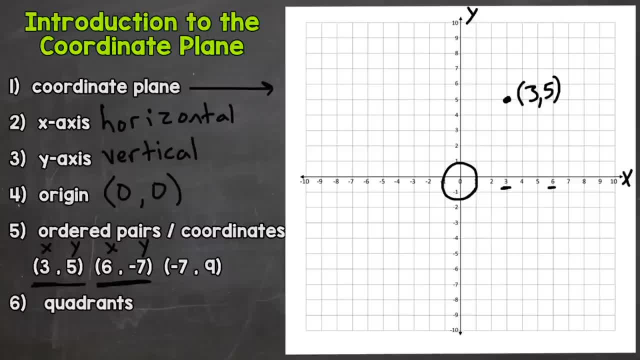 time we're going to go down seven, though, because that's a negative seven. So over six down to negative seven. plot a point where they intersect- I'm going to label this point as well. And then, lastly, we have negative seven, nine, So again X. 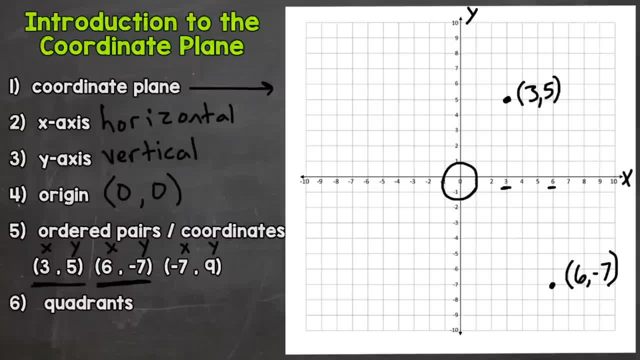 always comes first, followed by y. Now, this time we're going to go left of zero, because that's a negative seven. So negative seven is over here. and then our y is positive, a positive nine. So we're going to go up, Plot our point and I'll label negative. 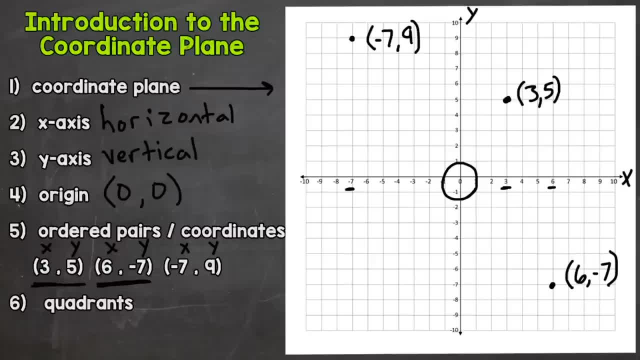 seven, nine, So again always side to side and then up or down. Lastly, we have quadrants. Now if you look at your coordinate plane there, you'll notice that we have four sections: top right, top left, bottom left, Bottom right. So this three, five right here, this top fourth, this is considered. 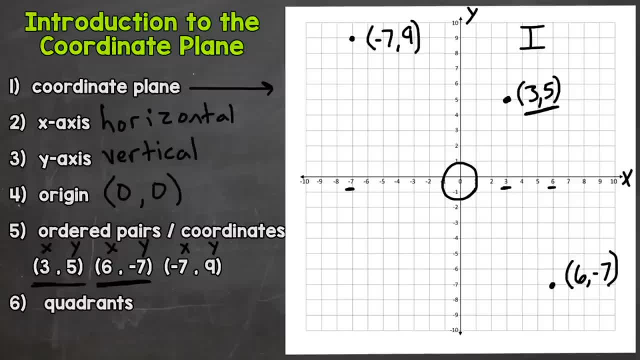 quadrant one. I'm going to use Roman numerals here. Now I'm going to jump to the left, where negative seven nine is. This is considered quadrant two. So negative seven nine. that point is plotted in quadrant two. Now we're actually going to go down to the bottom left, and that is quadrant three. 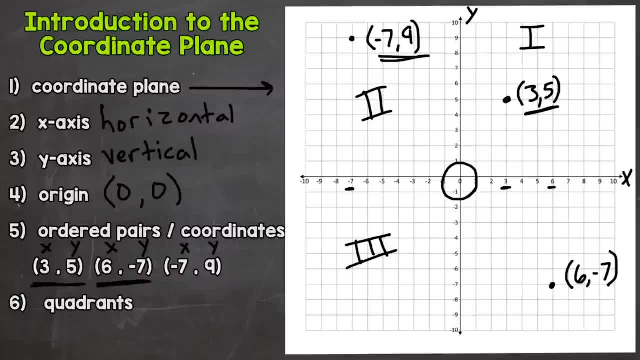 And then we go to the bottom right and that is quadrant four. So we actually go around this way when we count out our four quadrants. So again one, two, three and four, So six negative seven. That point is plotted in quadrant four.